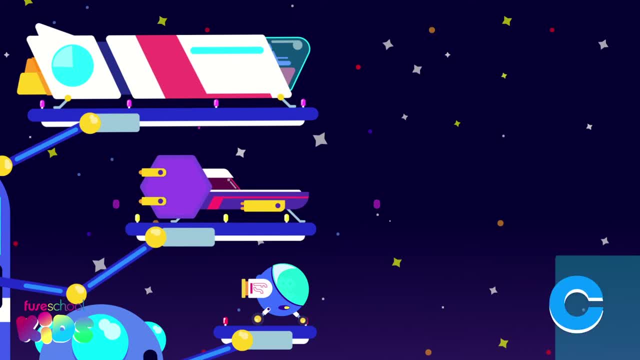 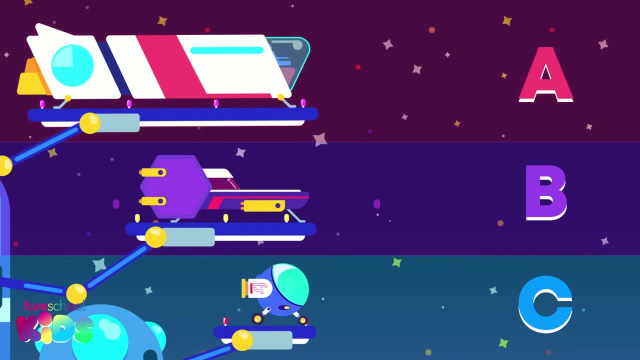 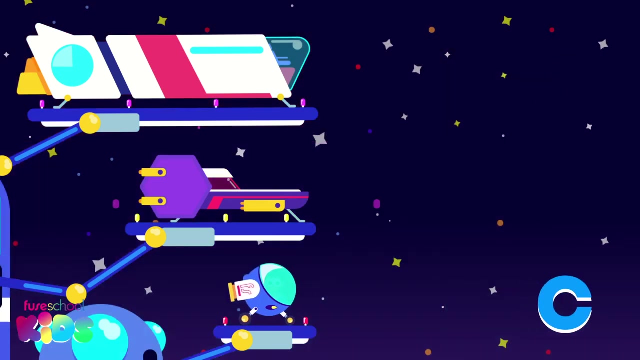 Which of these spaceships is the longest? If you said spaceship A, that's right, It is the longest because it is longer than the other spaceships. If I travelled in the shortest spaceship, which is mine, Well done to everyone who said spaceship C It is the shortest because it is shorter than the others. 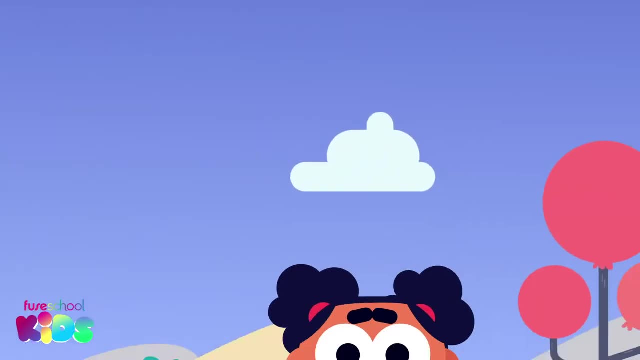 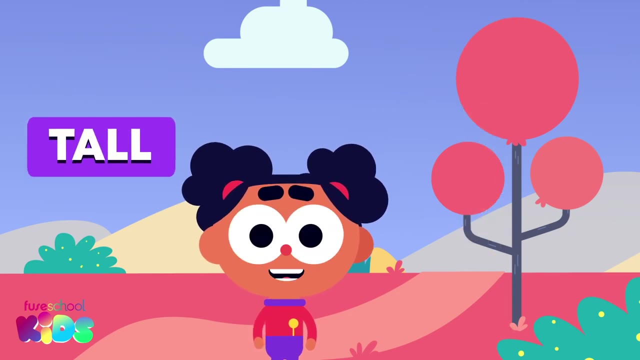 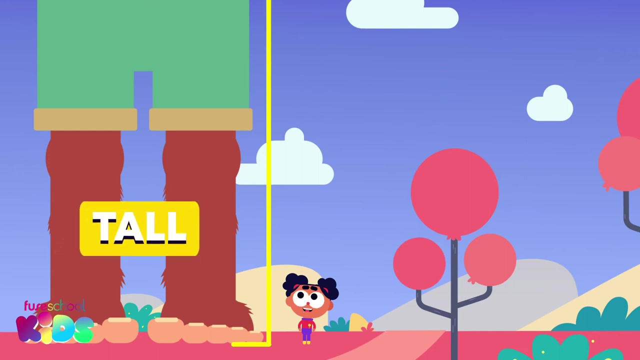 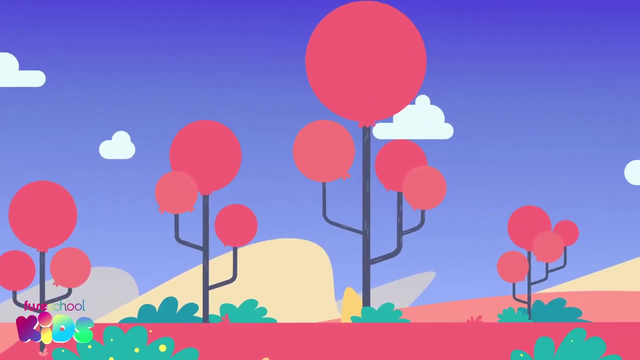 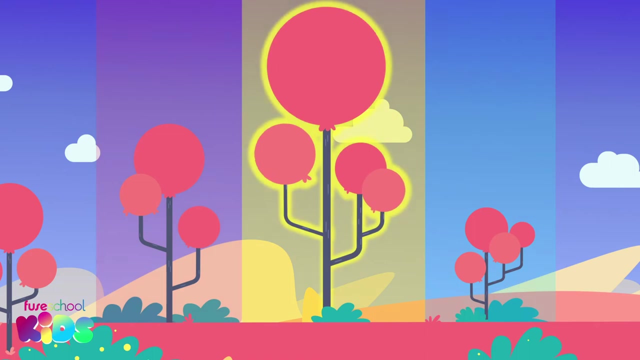 Let's explore Giant Planet. Height tells us how tall or high something is. We talk about height using the words tall and short. This giant is tall. I am shorter than him. He is taller than me. Can you see which of these is the tallest tree? 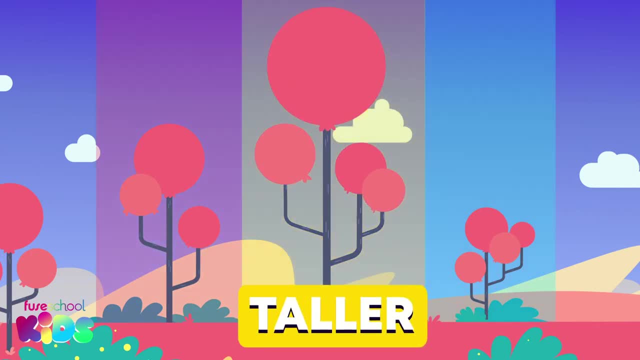 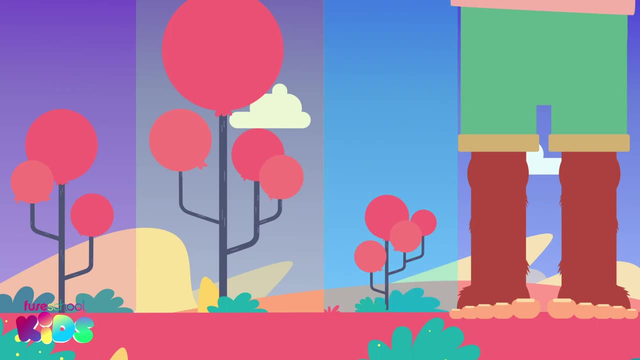 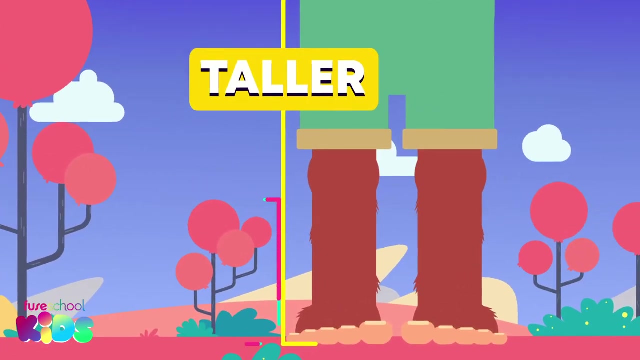 This tree is the tallest because it is taller than the others. Can the giant stand under the shortest tree? If you said no, that's right, The giant is taller than the shortest tree. He cannot fit under it because he is too tall. 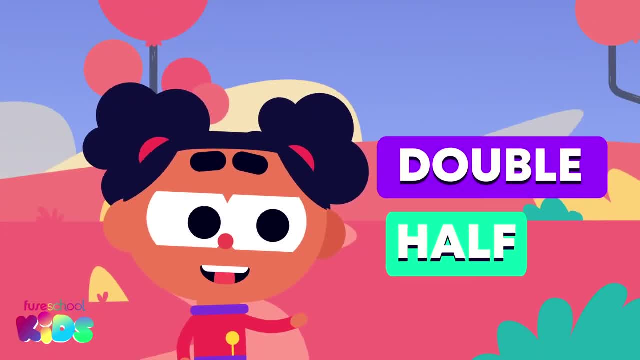 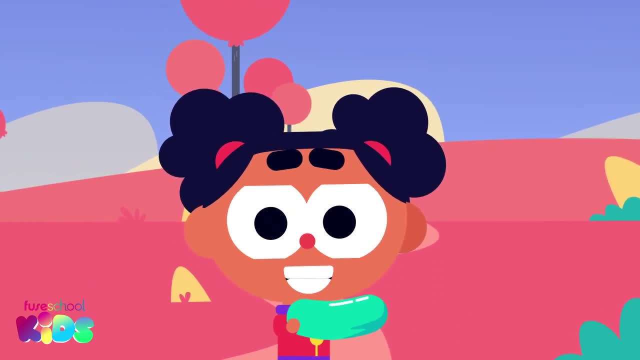 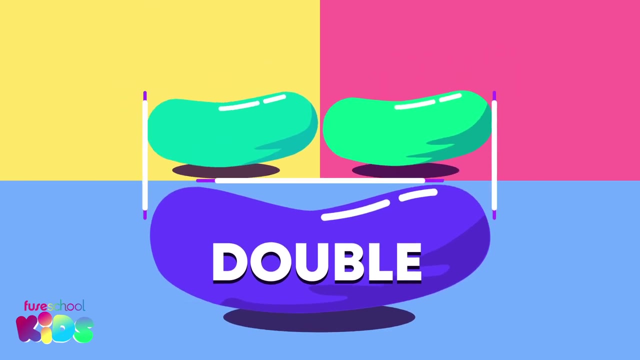 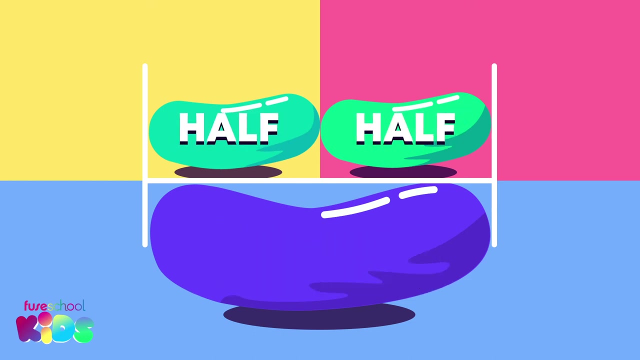 We can use double and half to describe length and height too. Look at the magic beans I got from Giant Planet. The purple bean is double the length of the other because it is as long as two green beans. Double means twice as many. The green bean is half as long as the purple bean because it only reaches half way. 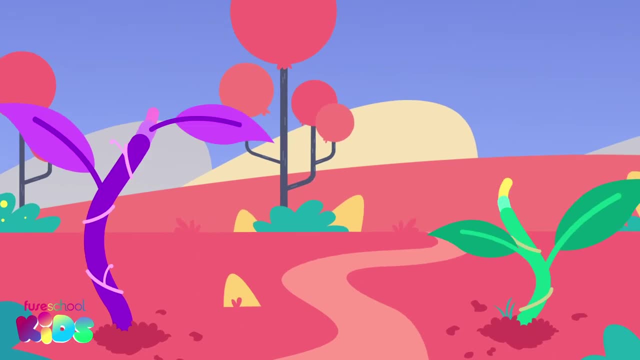 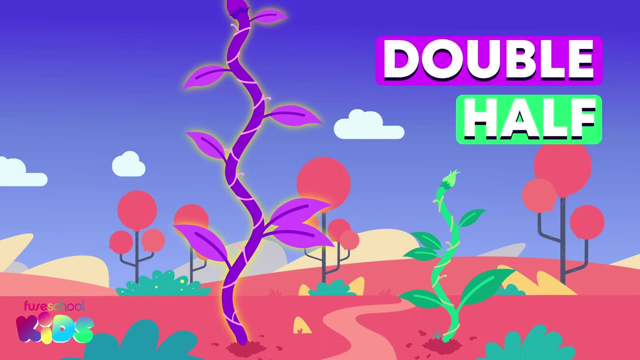 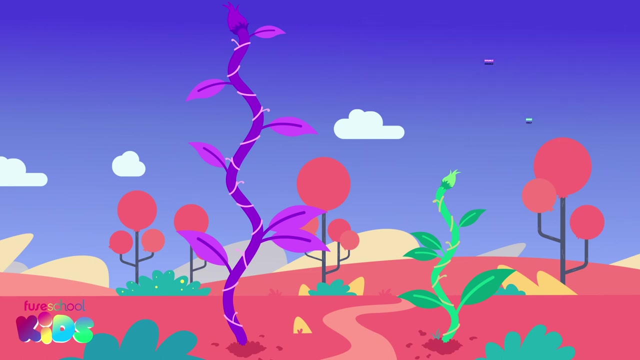 Look, my magic beans are starting to grow. Is this beanstalk double or half the height of the other? Double the height is right. It is double the height because it is as tall as two of them. What about this beanstalk? Is it double or half the height of the other?